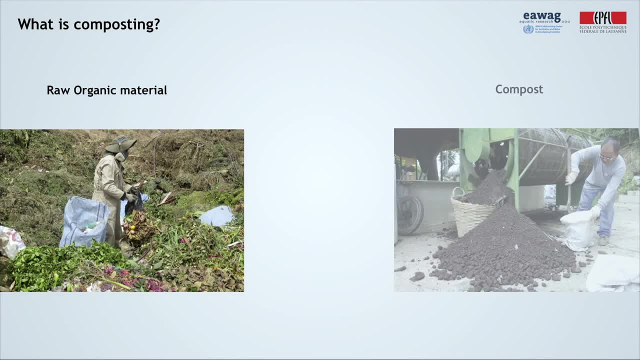 Composting is a controlled decomposition of raw organic material into biologically stable hammock substances, also called compost. This is carried out by microorganisms in the presence of oxygen. The final product, compost, is stable, doesn't degrade further and it can act as an excellent soil amendment. 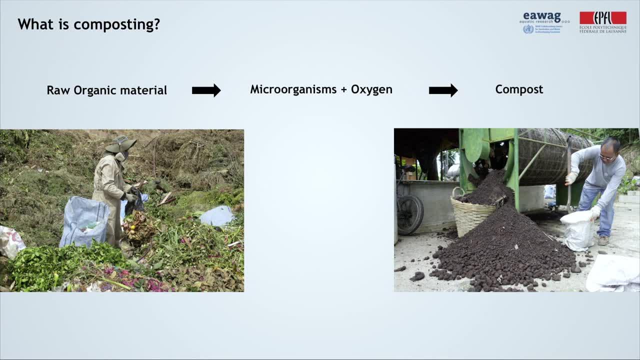 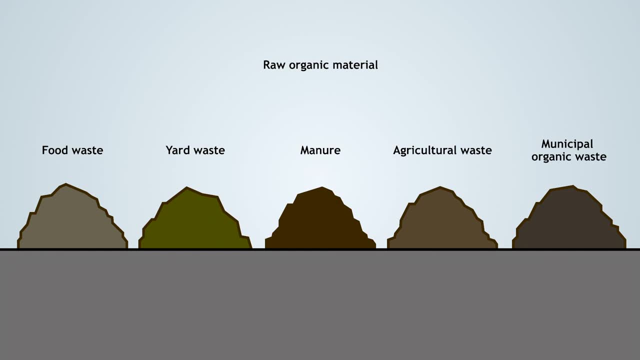 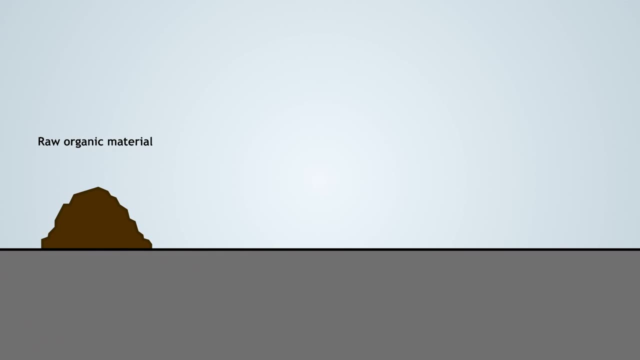 Let's now have a closer look to what exactly happens during composting. The first ingredient we need is raw organic material, such as food waste, jar waste, manure, agricultural waste, municipal organic waste, etc. These materials are broken down into smaller particles and are later piled up. 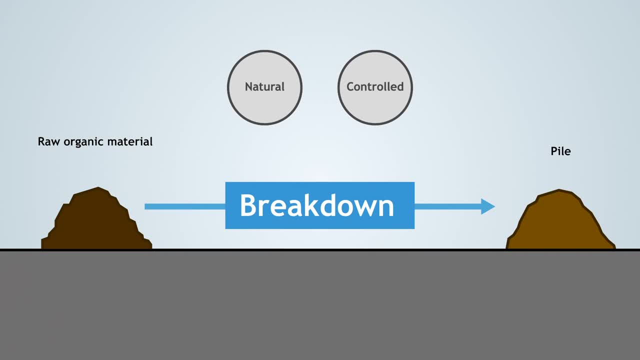 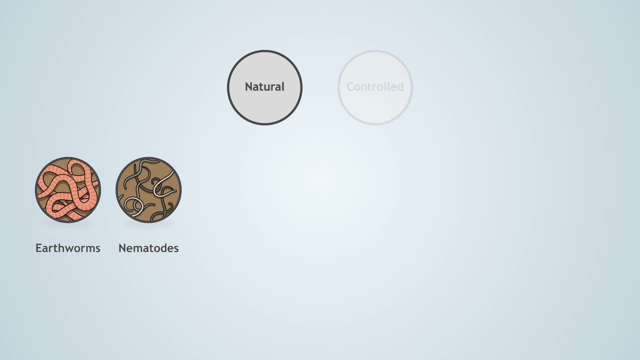 This breakdown can be known by the following: It can be natural or controlled. When natural, first the compost pile is made and then the breakdown happens, which is carried out by earthworms, nematodes and soil insects such as mites, sawbugs, springtails, ants and beetles. 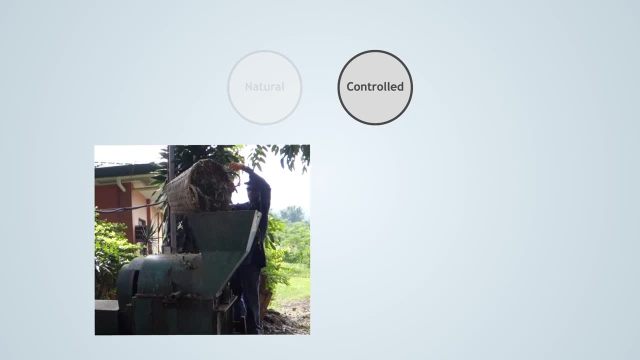 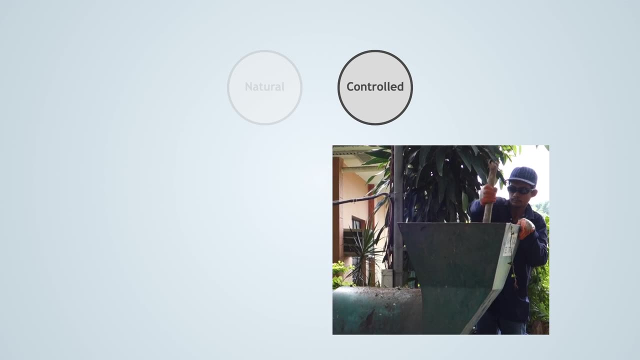 When controlled. first operators break down large particles through grinding, shredding or chopping, as shown in the video, and then they prepare the pile. Breakdown in this case is a preliminary step. Of course, the controlled breakdown is much faster than the natural breakdown. 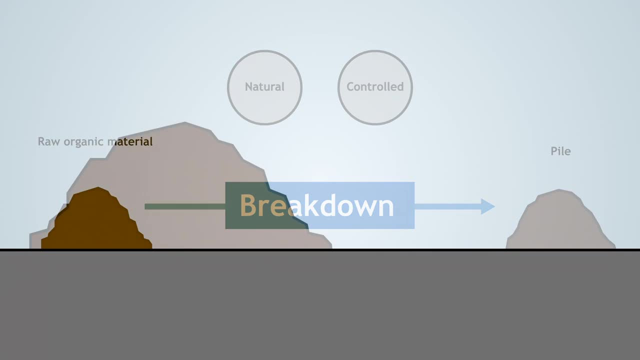 Once optimal physical conditions are established, microorganisms naturally found in soils colonize the organic material and initiate the decomposition process. Soil bacteria, fungi, actinomycetes and protozoa are the most commonly found microorganisms. The decomposition process can be divided into two phases: the active and the curing phase. 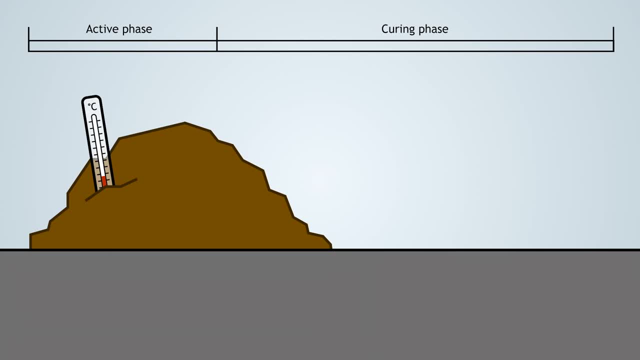 During the active phase, temperature increases rapidly due to the metabolism of microorganisms. In 24 and 72 hours, temperature can rise up to 55 to 70 degrees Celsius. This temperature increase hygienizes the material by killing pathogens. It also contributes to eliminate weed seeds and it breaks down phytotoxic compounds. 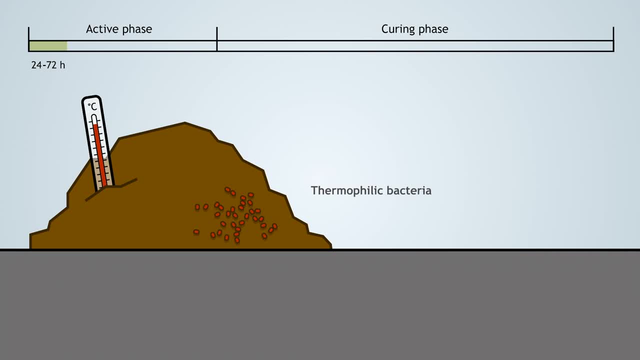 Under these conditions, thermophiles- those microorganisms that function at temperatures higher than 41 degrees Celsius- take over the decomposition activity. The active phase normally goes on for several weeks. During this time, oxygen and water need to be replenished in order to ensure the activity of the microorganisms. 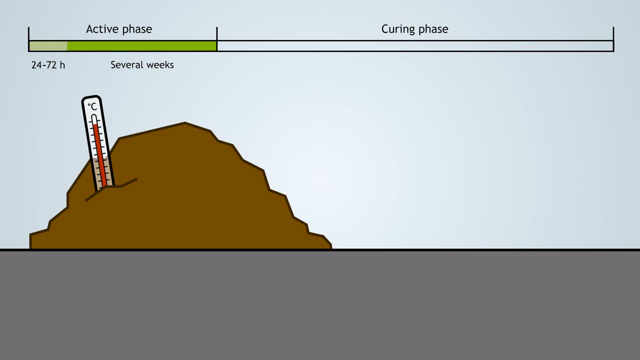 Once all the easily degradable or digestible materials are eaten, the activity of the thermophiles will drop And the curing phase starts. This is characterized by a temperature drop to 37 degrees Celsius. Oxygen consumption also drops and mesophilic bacteria recolonize the pile. 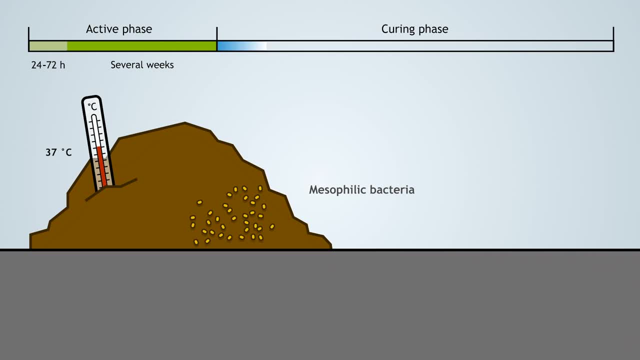 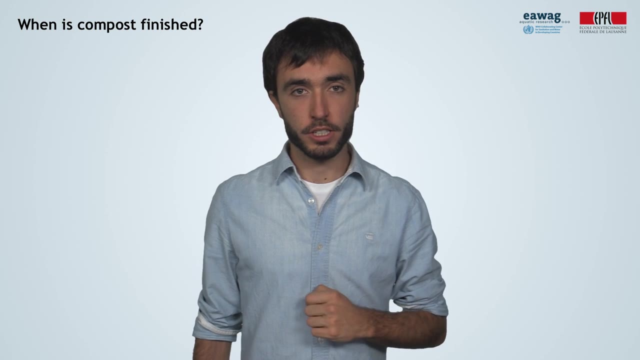 The decomposition of organic materials continues into stable hammock substances. There is no clearly defined time for curing. It can take as long as one month to one year, depending on feedstocks, composting method used and management. How do we know when compost is finished? 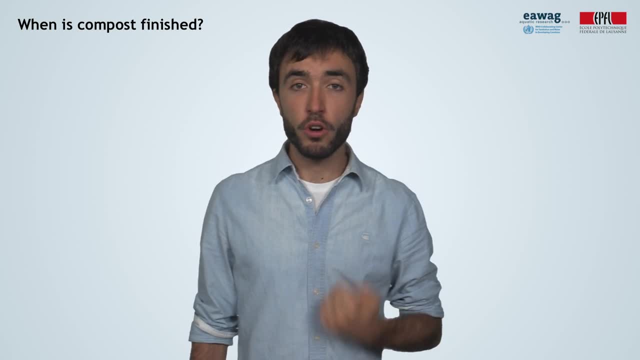 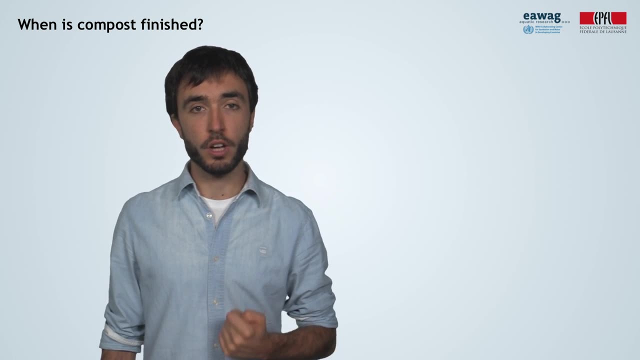 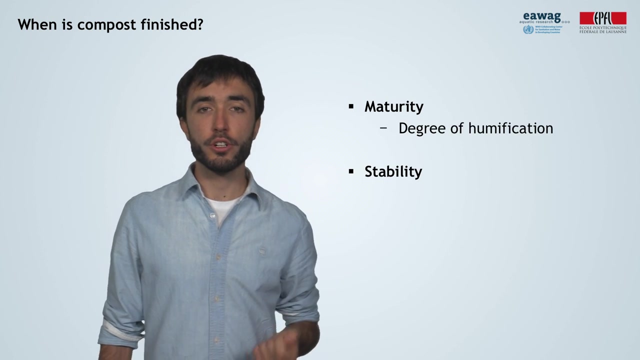 Compost is considered finished when the raw feedstocks are no longer actively decomposing and are biologically and chemically stable. The parameters that are used for this purpose are maturity and stability. Maturity is usually defined as the degree of humification conversion of organic compounds to hammock substances. 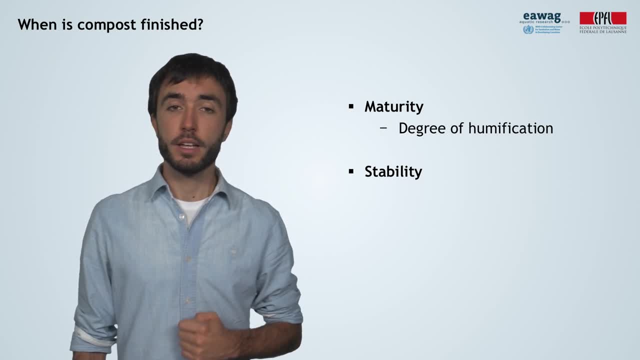 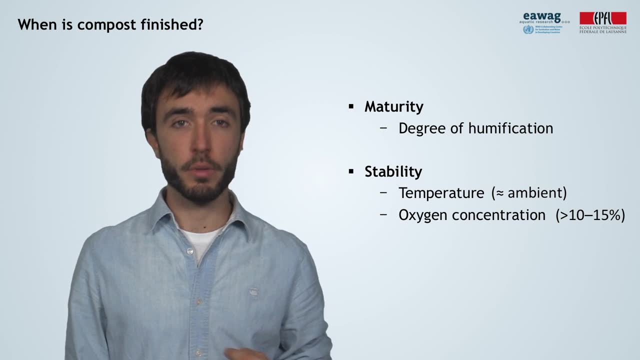 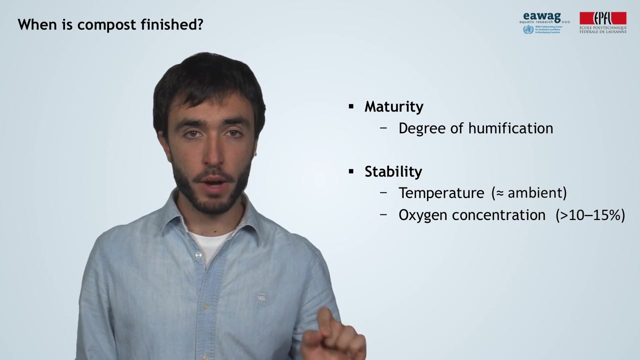 which are most resistant to microbial breakdown. Stability, on the other hand, is indicated by temperature and oxygen consumption. Measuring compost stability is normally easier than measuring maturity. The most clear indication of a stable or finished compost pile is when the temperature at the center of the pile returns to near ambient. 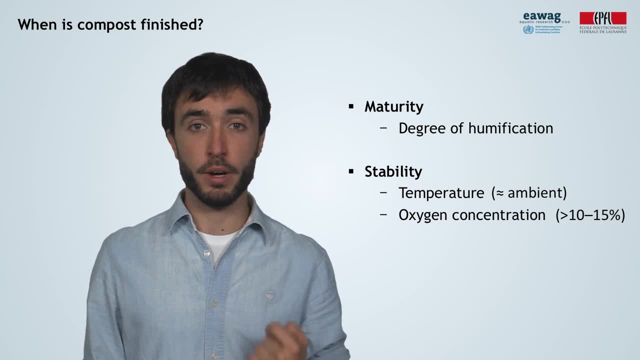 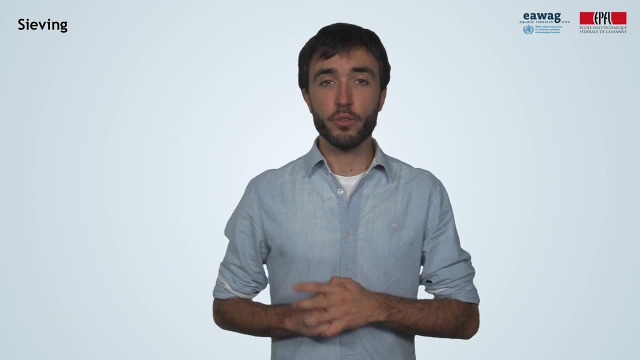 and when the oxygen concentrations in the air cavities inside the pile remain greater than 10% for several days. Once the curing phase is over. depending on the final use of compost and the origin of the organic material, the operators might want to separate possible impurities. 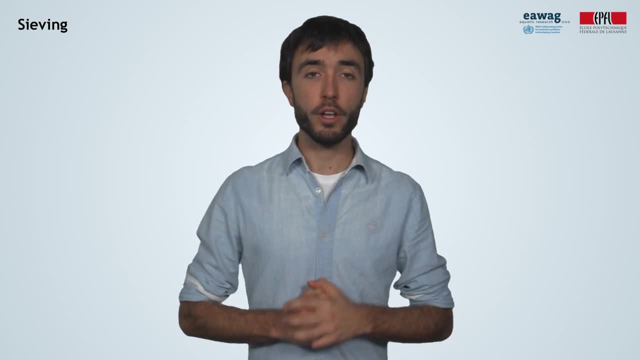 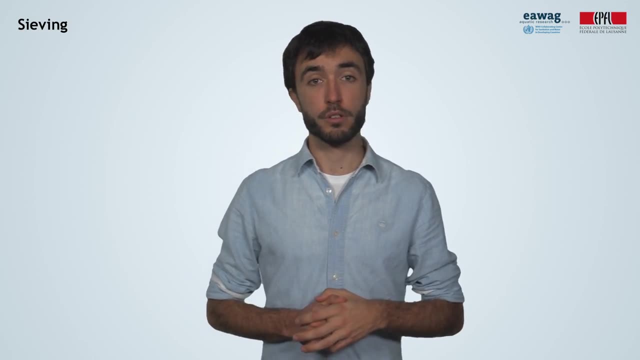 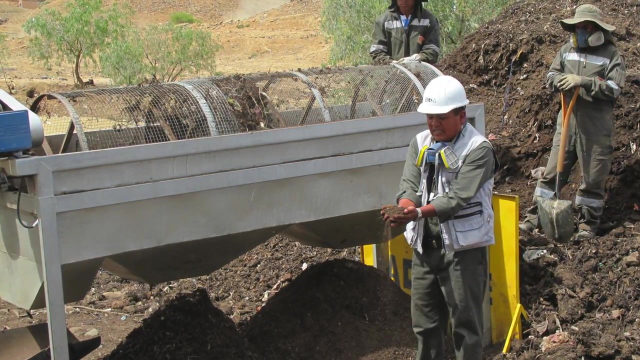 plastics or metals, or oversized and not fully composted chunks of organic waste. This is done by sieving the matured compost. Sieving or screening usually takes place before or after the curing phase. It is used for two purposes: To separate impurities and to produce a range of product grades suitable for various end uses. 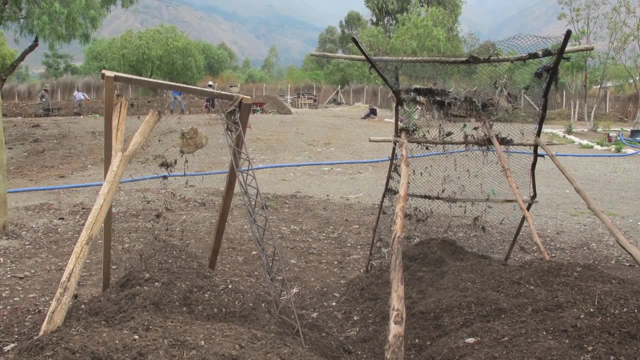 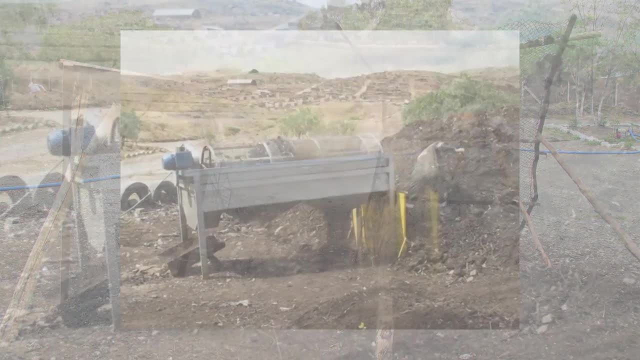 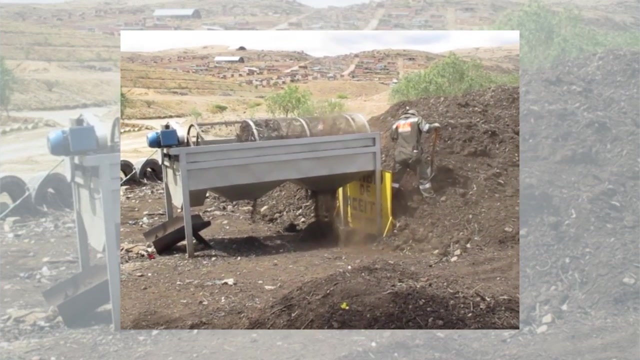 such as soil conditioning, mulching or others. Often, the organic oversize is fed back into the processing system so that they break down fully. There are engine-driven sieves as well as more simple and low-tech sieves, As long as they accomplish their goal of diverting impurities and separating the compost into different particle sizes.